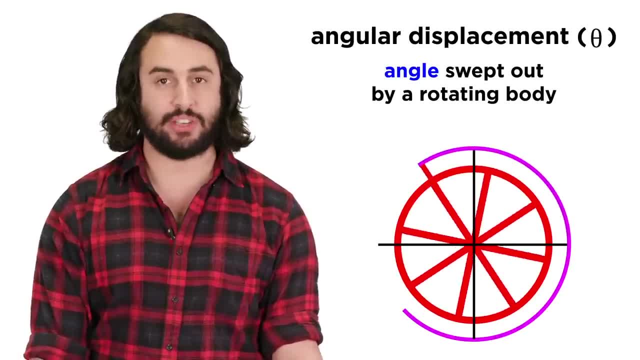 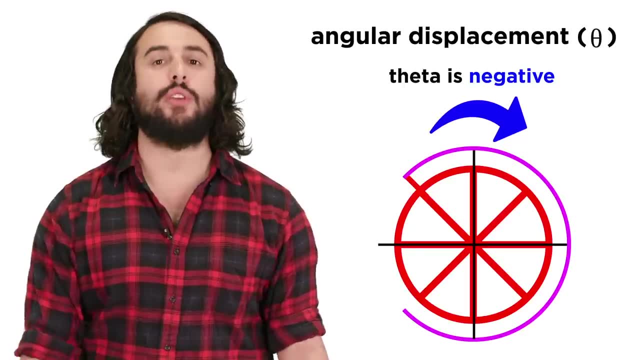 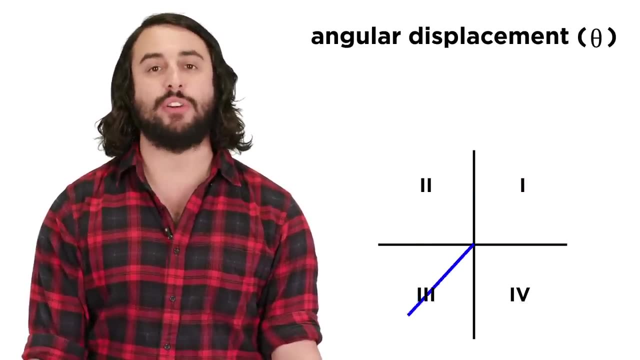 through a rotating body that intersects the axis of rotation. This value will be positive if the motion is counterclockwise and negative if it is clockwise. If you have a hard time remembering this, just remember that in going counterclockwise around the xy plane, we will cover quadrants one, two, three and then four. so positive: 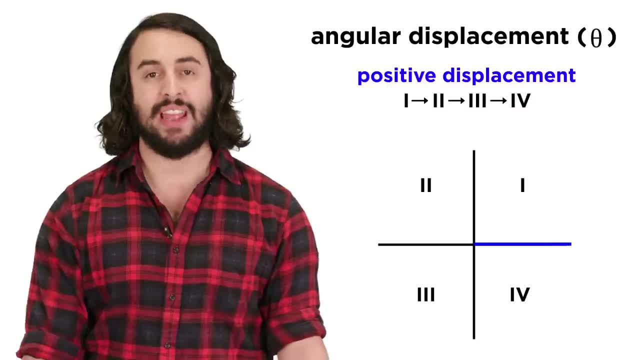 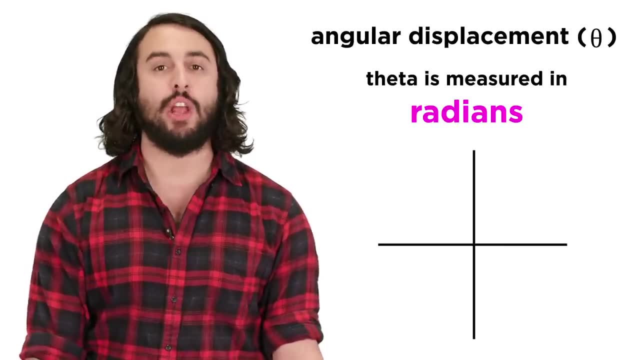 angular displacement correlates with a positive increase in the number quadrant that is being traversed over time. The SI unit for angular displacement will not be degrees, but rather radians. We will discuss the derivation and importance of the radian in the next section. Thank you for watching. 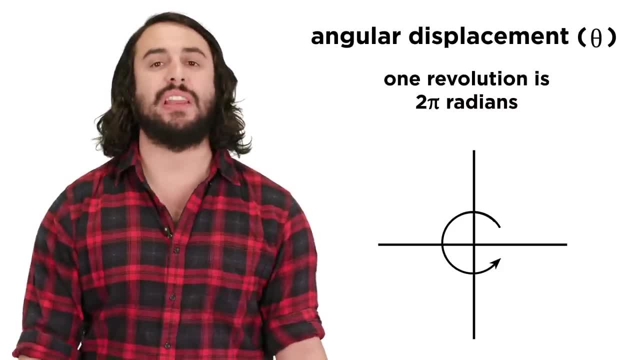 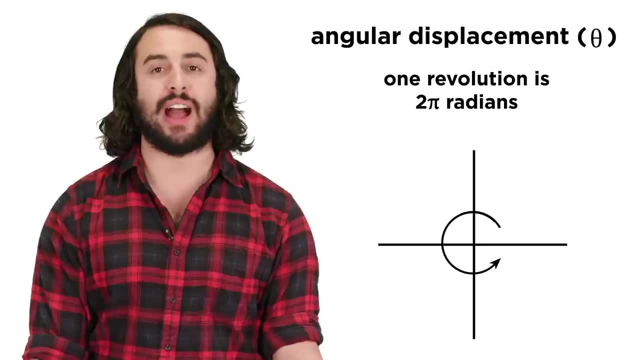 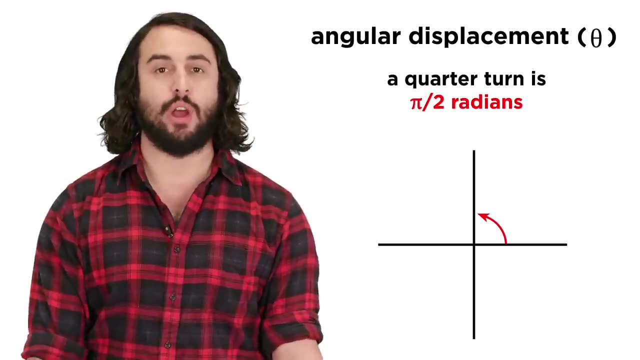 In the upcoming mathematics course. But for now we simply need to know that one full revolution is equal to two pi radians. So if the rotation completed by the object is a counterclockwise quarter turn, the angular displacement is one half pi radians or pi over two. 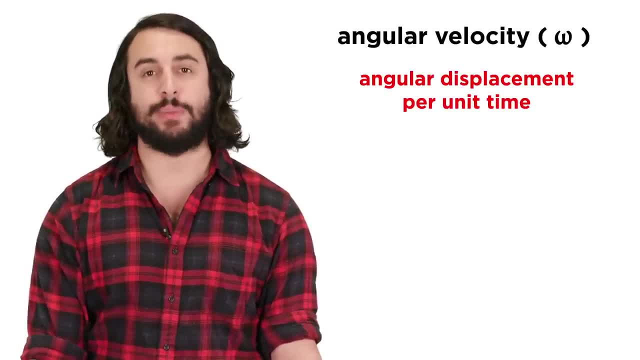 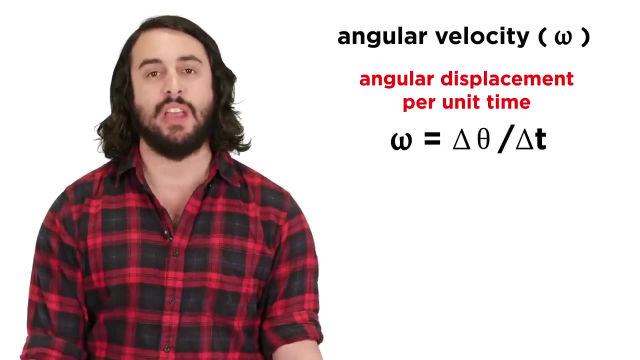 Angular velocity, as one might expect, is equal to the angular displacement over some time period, just the same way that linear velocity is equal to linear displacement over time. The average angular velocity, represented by the Greek letter omega, is therefore given as delta theta over delta t. 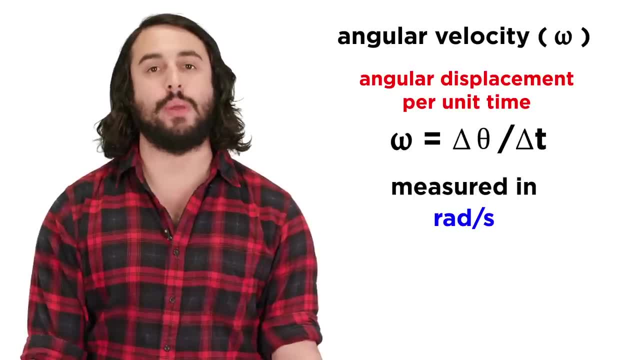 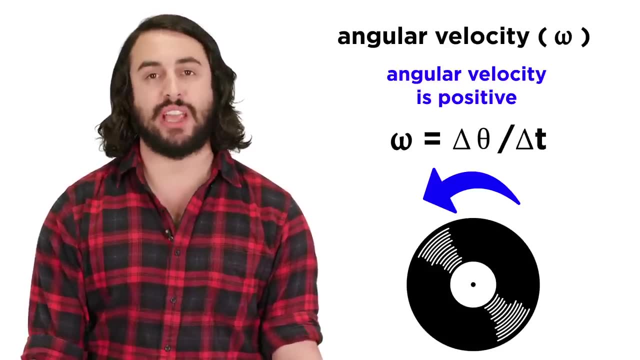 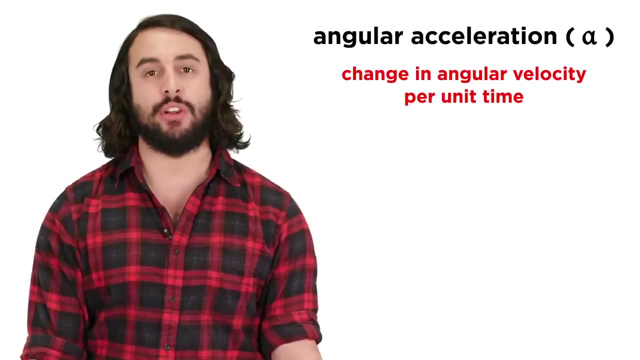 The SI unit for this value will be radians per second, although we will frequently encounter other units like revolutions per minute or rpm. Again, counterclockwise rotation involves positive angular velocity and clockwise will be negative. Lastly, angular acceleration, represented by the Greek letter alpha, is equal to the 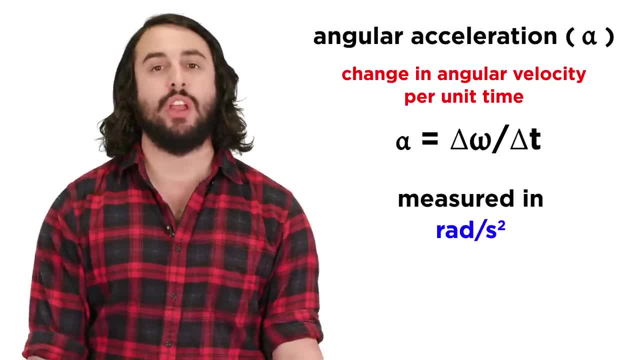 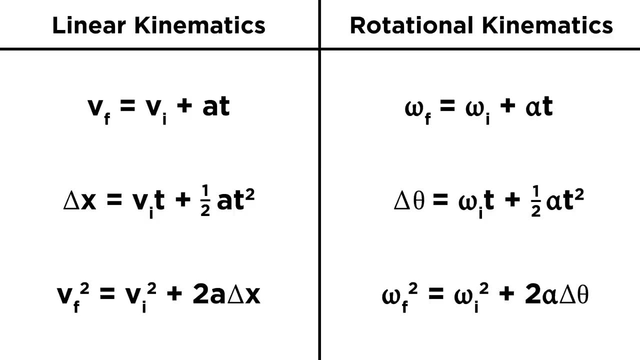 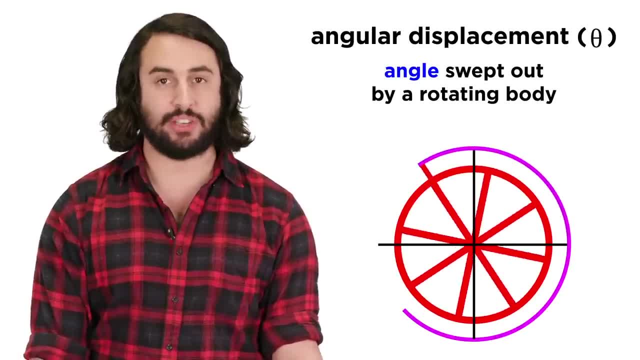 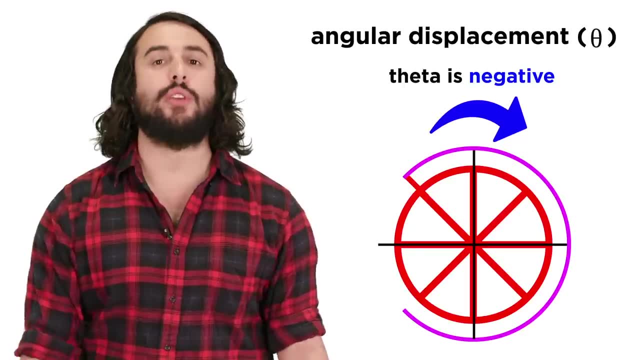 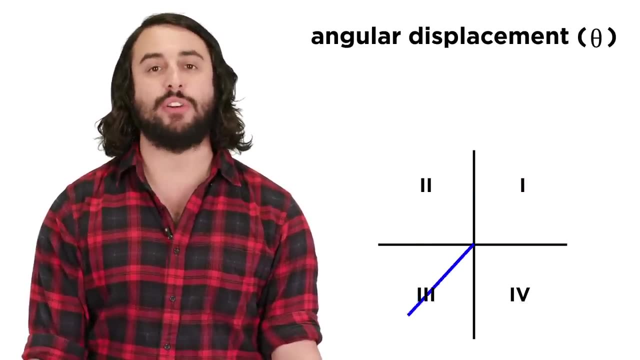 through a rotating body that intersects the axis of rotation. This value will be positive if the motion is counterclockwise and negative if it is clockwise. If you have a hard time remembering this, just remember that in going counterclockwise around the xy plane, we will cover quadrants one, two, three and then four. so positive: 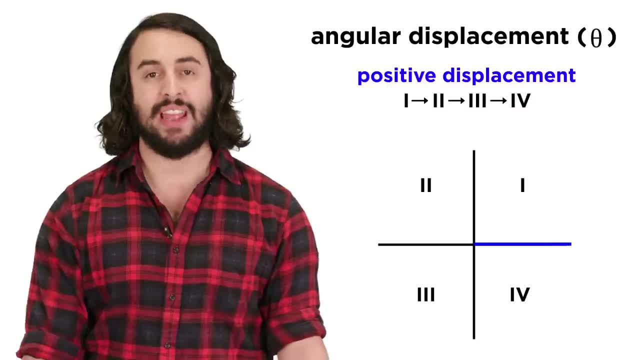 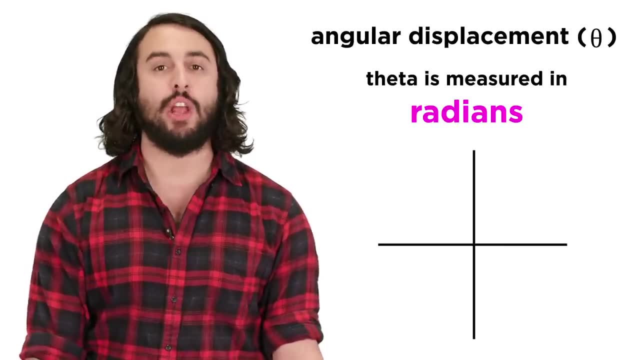 angular displacement correlates with a positive increase in the number quadrant that is being traversed over time. The SI unit for angular displacement will not be degrees, but rather radians. We will discuss the derivation and importance of the radian in the next section. Thank you for watching. 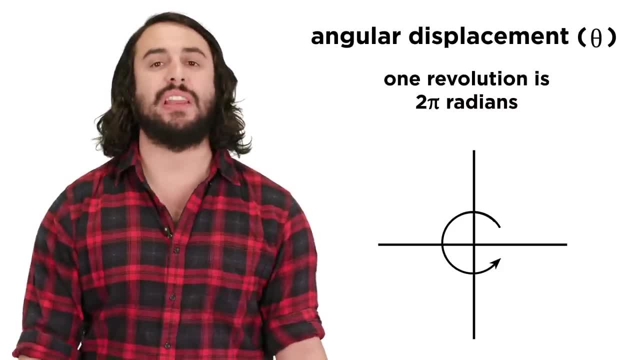 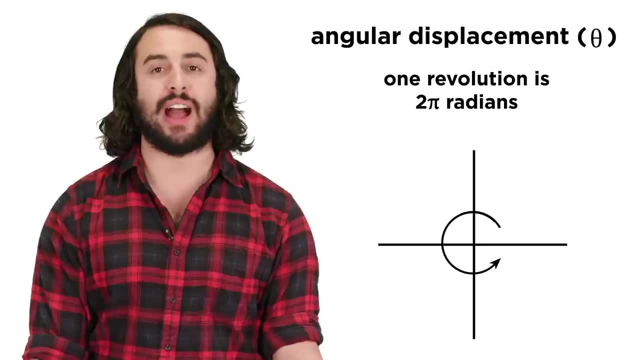 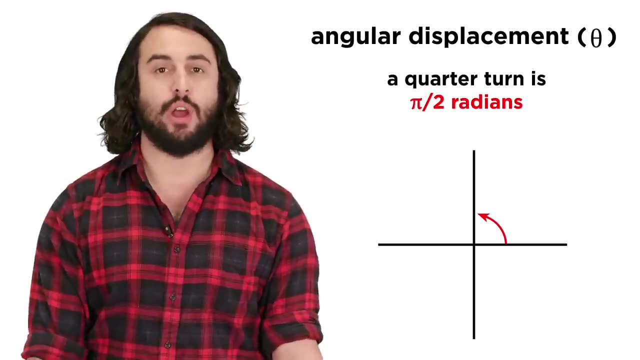 In the upcoming mathematics course. But for now we simply need to know that one full revolution is equal to two pi radians. So if the rotation completed by the object is a counterclockwise quarter turn, the angular displacement is one half pi radians or pi over two. 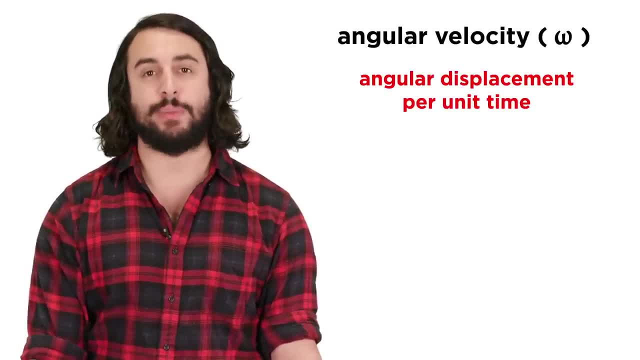 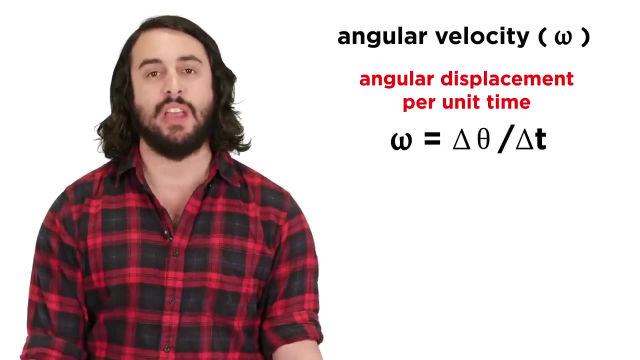 Angular velocity, as one might expect, is equal to the angular displacement over some time period, just the same way that linear velocity is equal to linear displacement over time. The average angular velocity, represented by the Greek letter omega, is therefore given as delta theta over delta t. 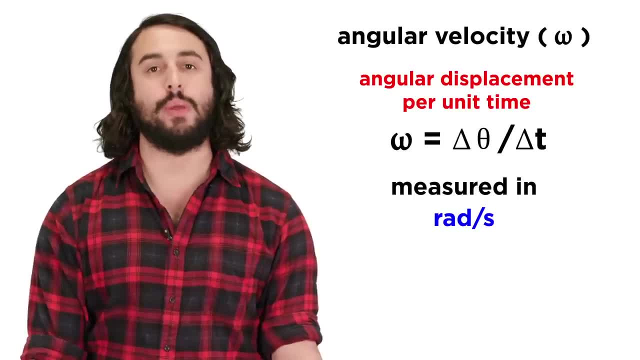 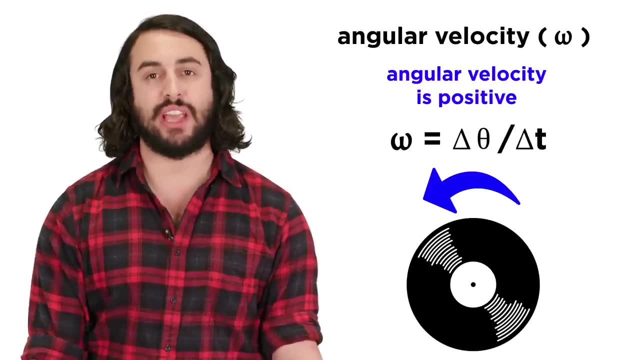 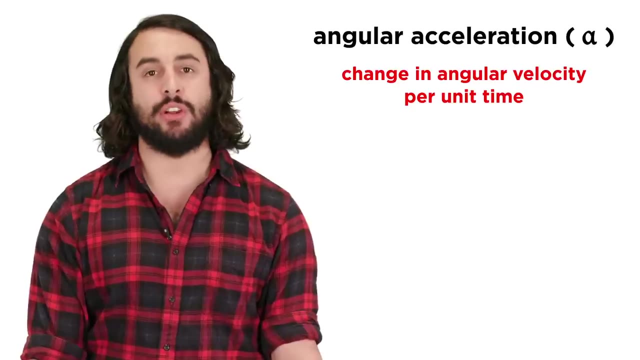 The SI unit for this value will be radians per second, although we will frequently encounter other units like revolutions per minute or rpm. Again, counterclockwise rotation involves positive angular velocity and clockwise will be negative. Lastly, angular acceleration, represented by the Greek letter alpha, is equal to the 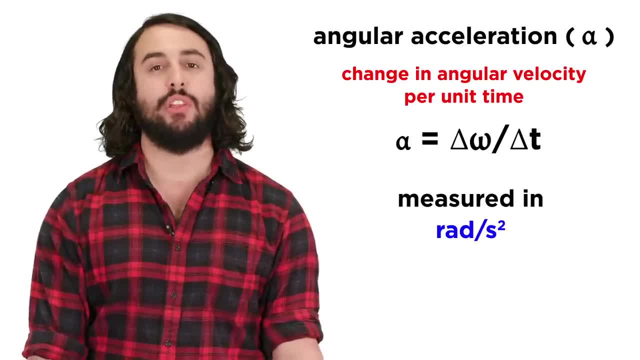 change in angular velocity over time. So if you have a hard time remembering this, just remember that in going counterclockwise there is a change in angular velocity over some time period. This will be equal to delta omega over delta t, with units of radians per second squared. 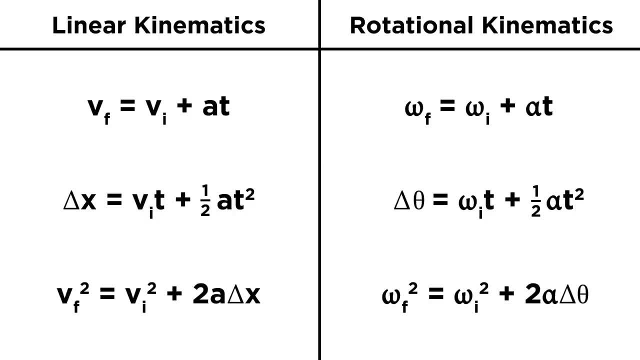 Now that we have defined these terms, we can begin to understand that rotational kinematics will utilize equations that are direct analogs of those involved with linear kinematics. We just swap out linear components for angular ones. Looking at these familiar equations, if we just exchange, 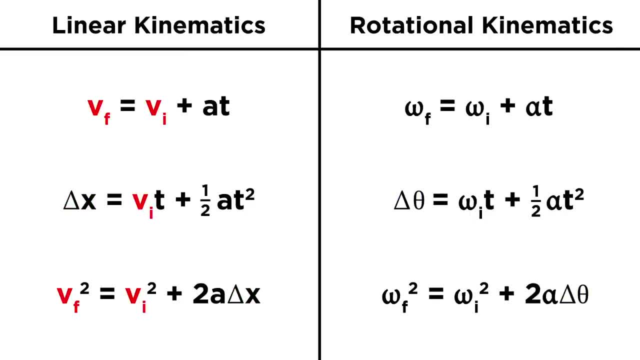 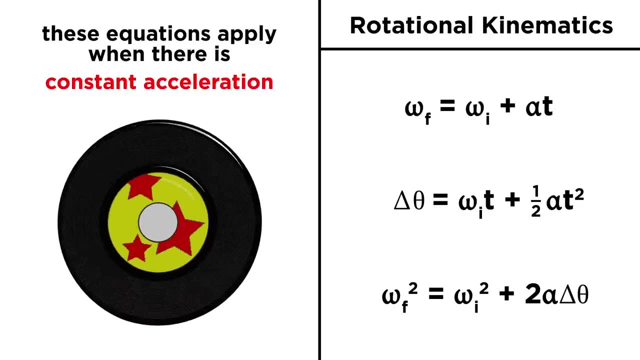 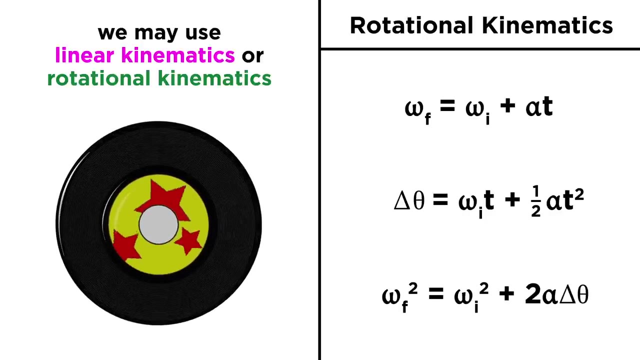 displacement- for angular displacement, velocity for angular velocity, and acceleration- for angular acceleration. we arrive at a new set of equations that allow us to calculate rotational motion, and they will apply to any system with rotational motion under constant angular acceleration. Depending on the scenario, it may or may not be easier to model rotational motion with 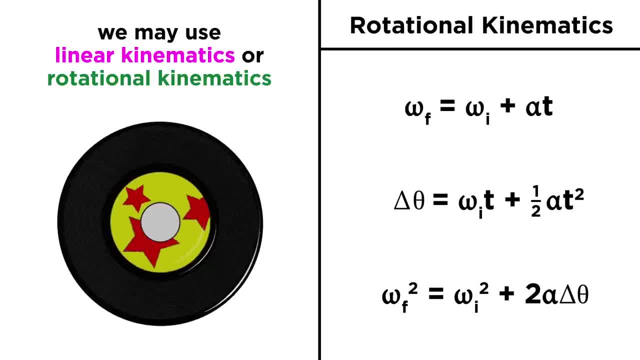 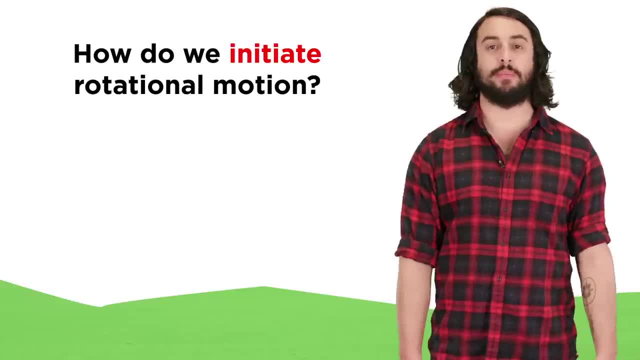 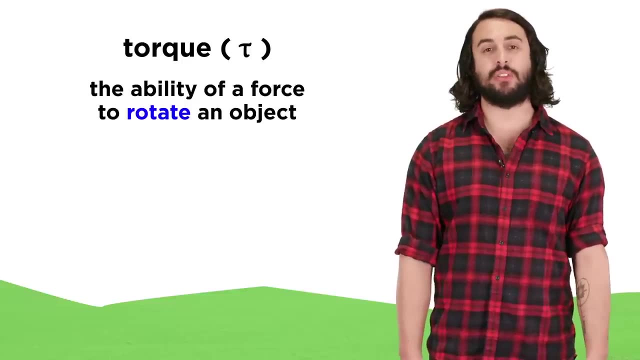 these equations rather than with the linear ones, Where we have to use tangential velocities that vary according to the radius. How can we set a system into rotational motion? We can do this by generating something called a torque. Torque is defined as the ability of a force to rotate an object around some axis, whether 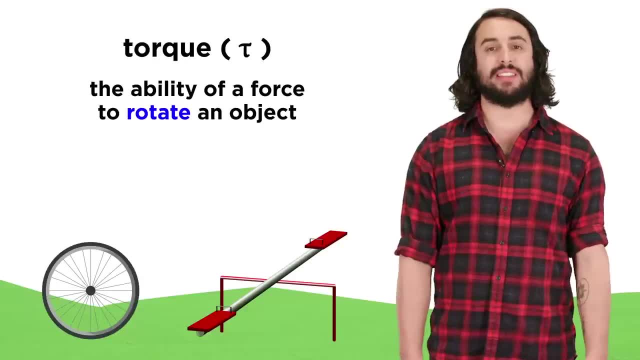 we are looking at a wheel, a seesaw or anything else that exhibits this kind of motion, And for now we can just look at a top-down view of a panel attached to a rod. And for now we can just look at a top-down view of a panel attached to a rod. 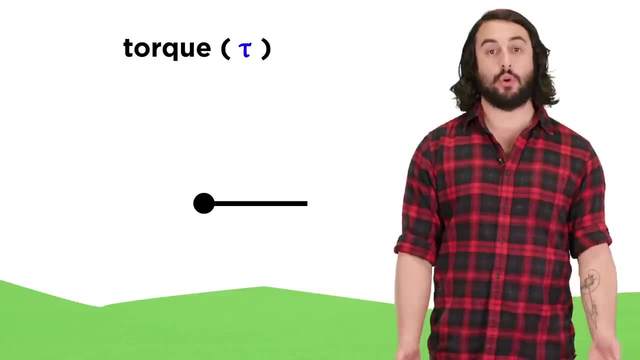 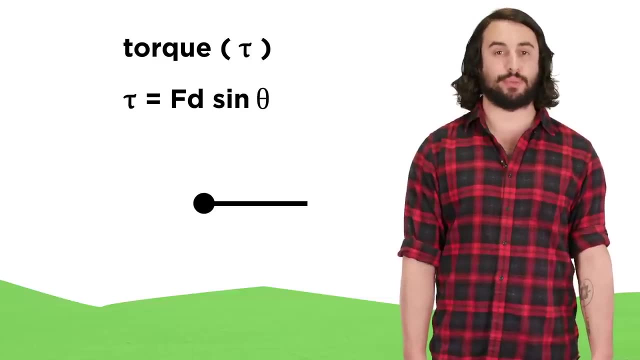 And for now we can just look at a top-down view of a panel attached to a rod. Torque, represented by the Greek letter tau, will be equal to the applied force times the distance over which the force is applied, times sine theta, where theta is the angle. 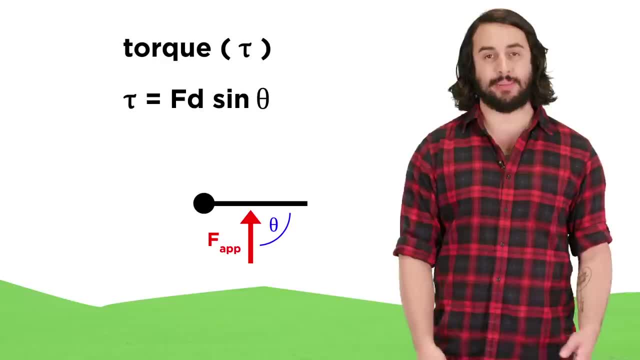 between the force vector and the plane of the rotating object. Torque will therefore have units of newton meters and torque will be at a maximum when the applied force is perpendicular to the plane containing the object, because the sine of ninety degrees is complete. with that, much of the applied force that is applied, whether 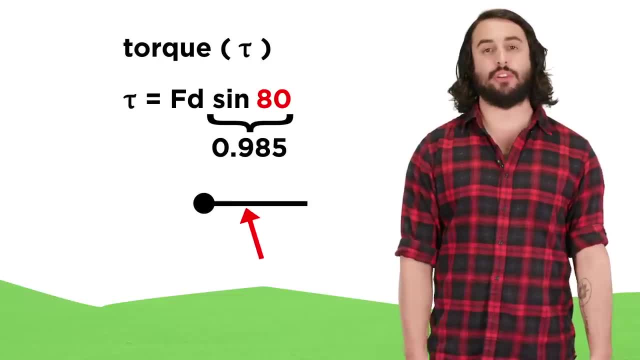 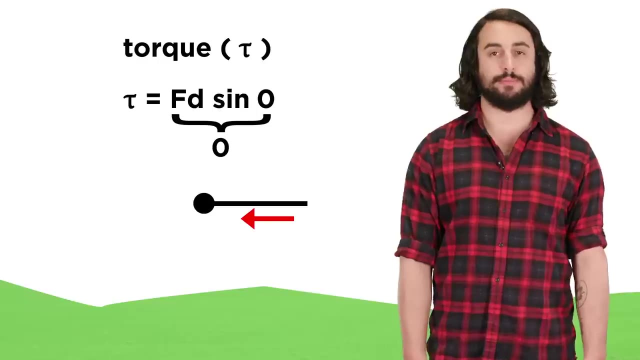 is 1.. Any angle less than 90 in either direction will give a sine value that is less than 1 and will therefore diminish the torque while still producing some motion until the angle is 0, at which point the whole expression will be equal to 0 and no motion can result. By convention, we will say that torque is 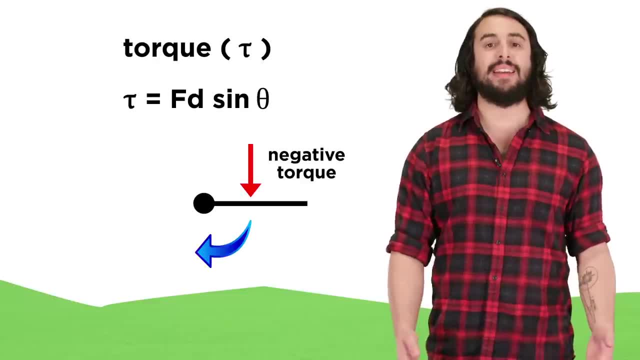 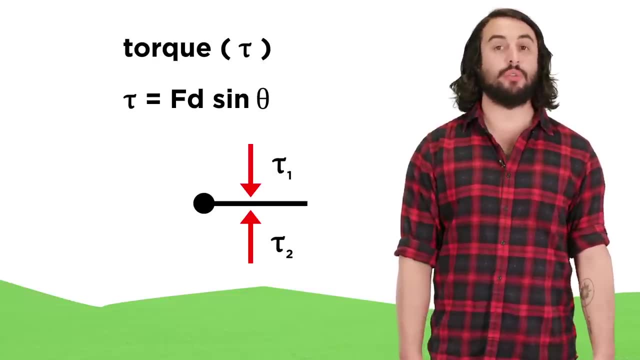 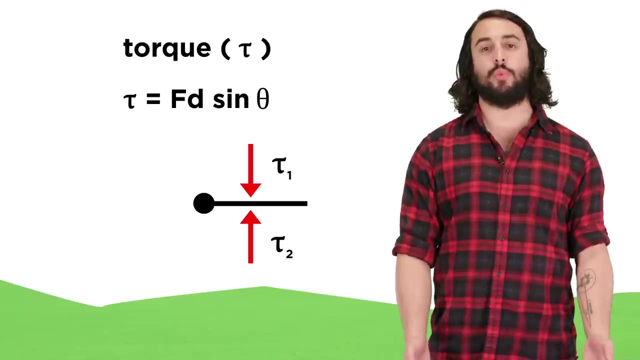 positive if it results in counterclockwise rotation and negative if it results in clockwise rotation as we are by now familiar. This must be the case because if two different forces act upon this object to produce opposite torques that are equal in magnitude, the object will not move and the sum of the 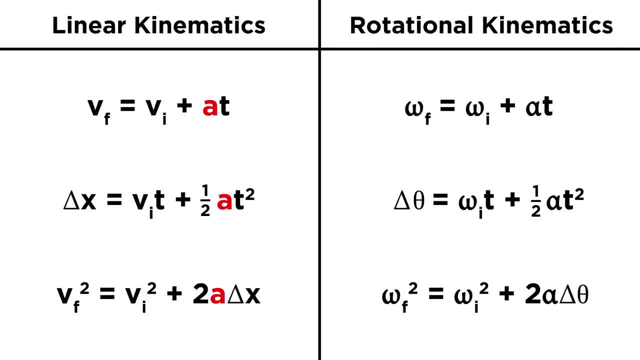 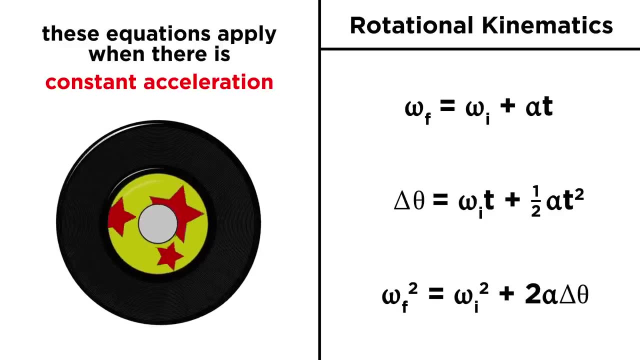 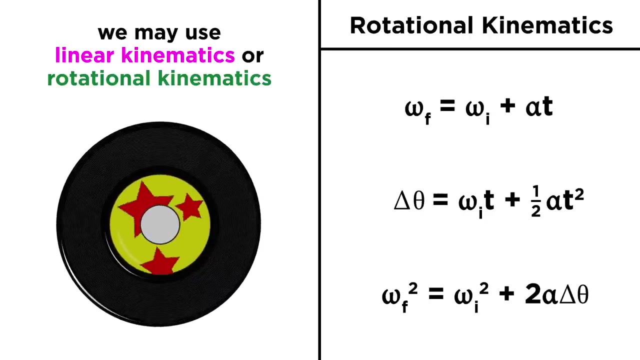 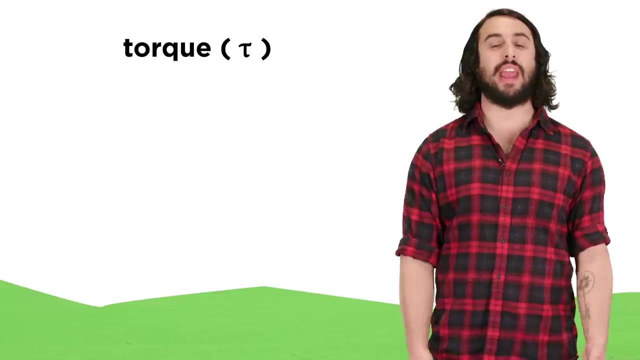 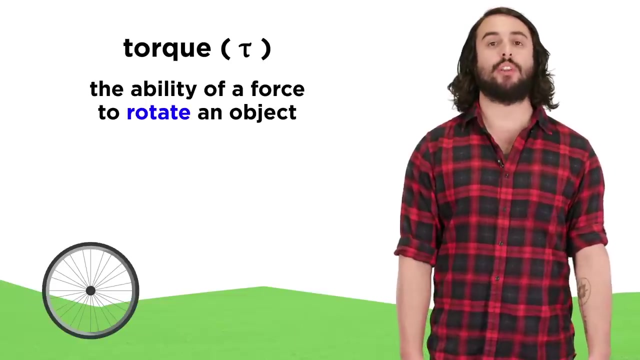 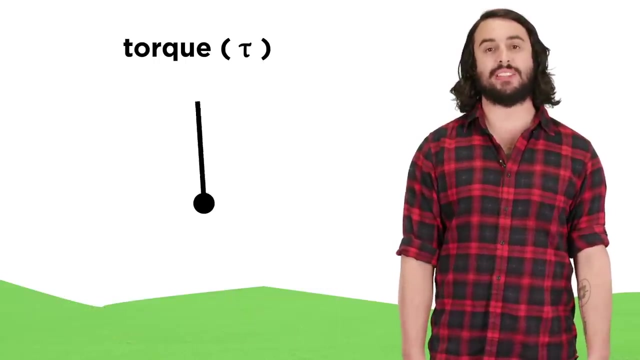 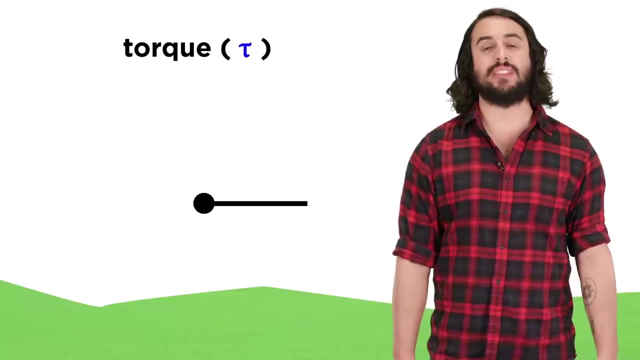 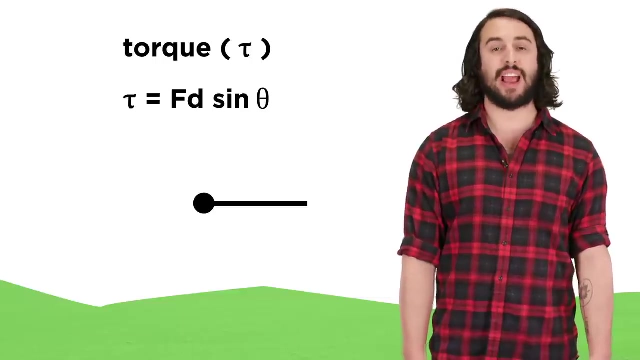 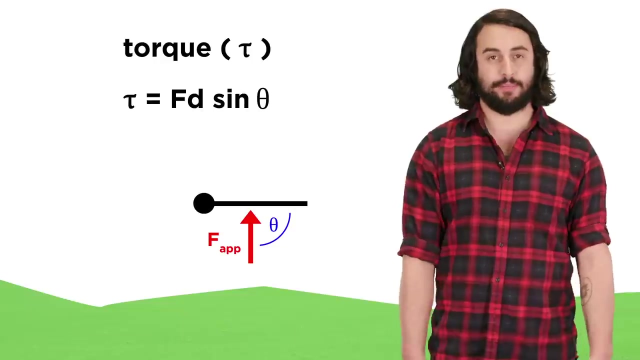 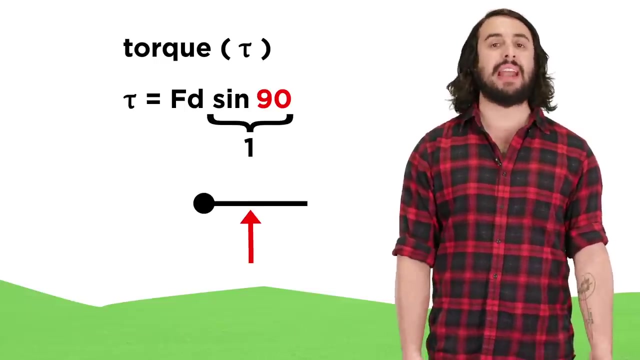 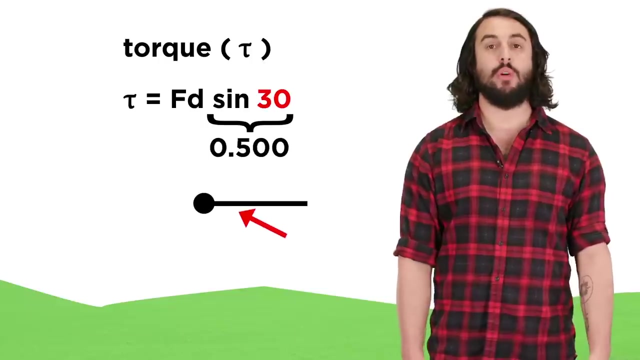 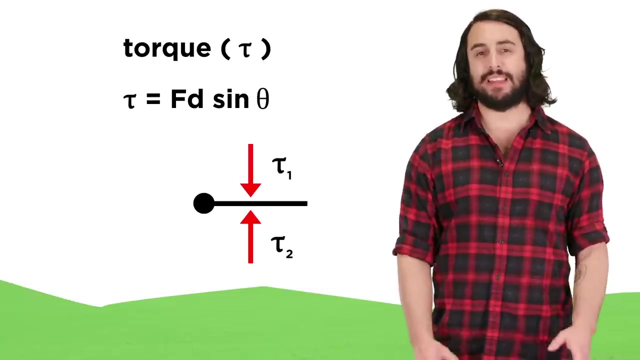 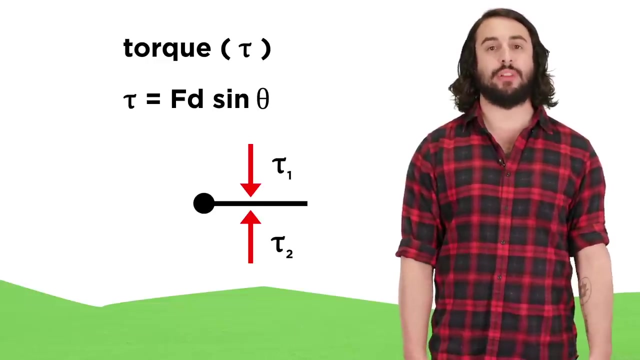 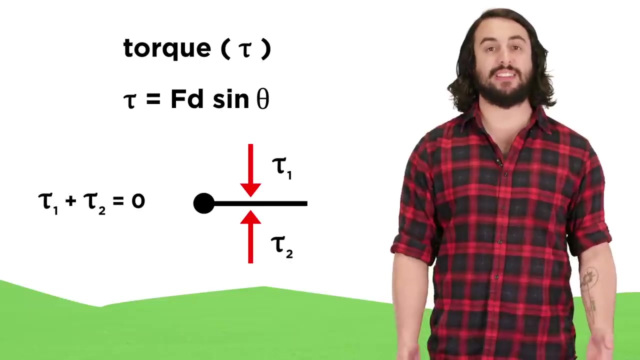 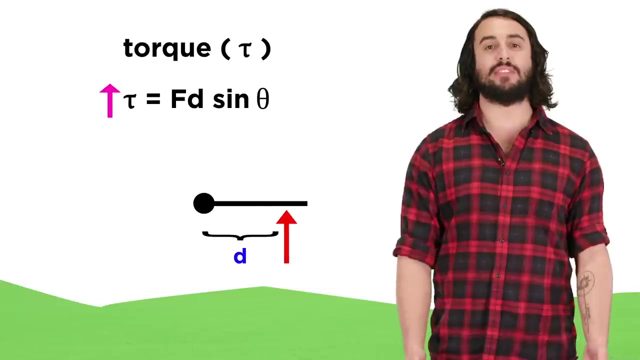 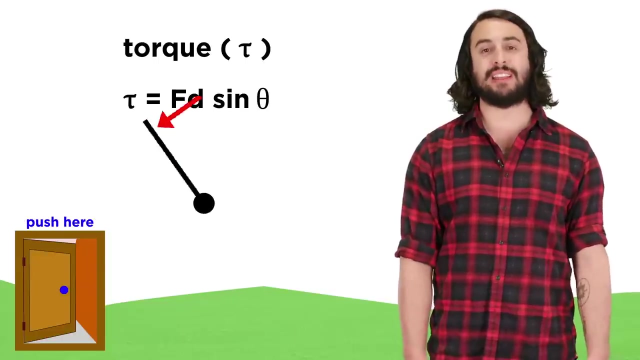 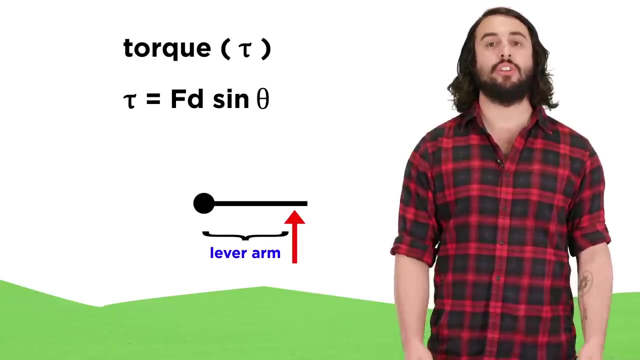 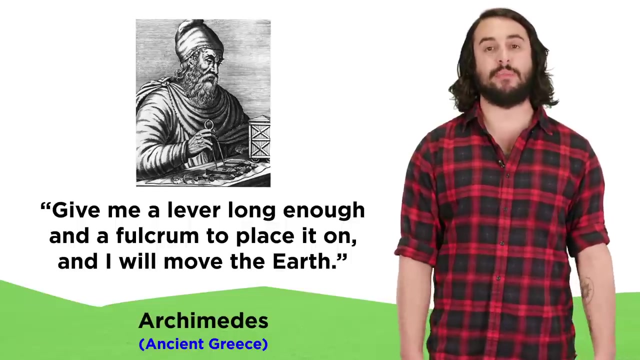 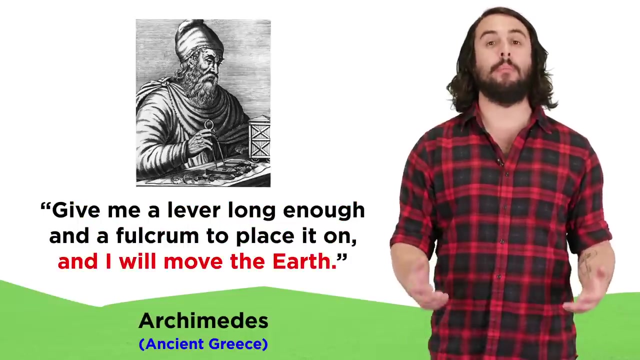 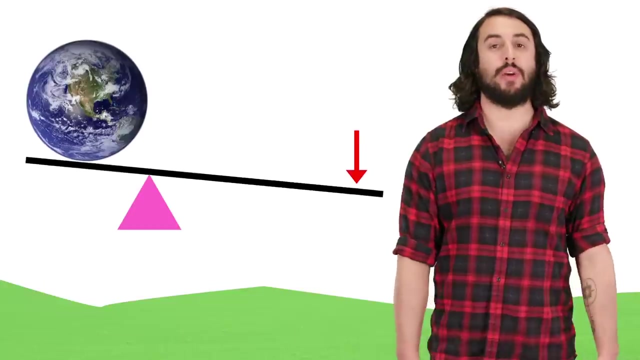 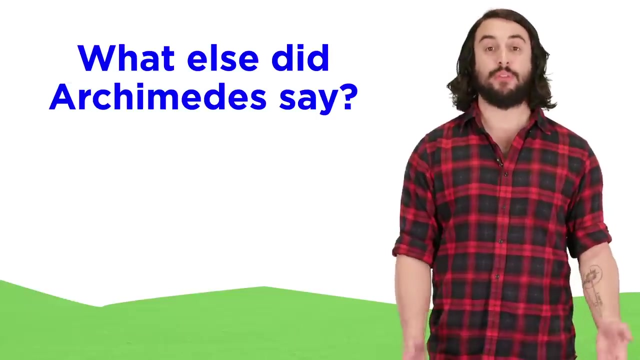 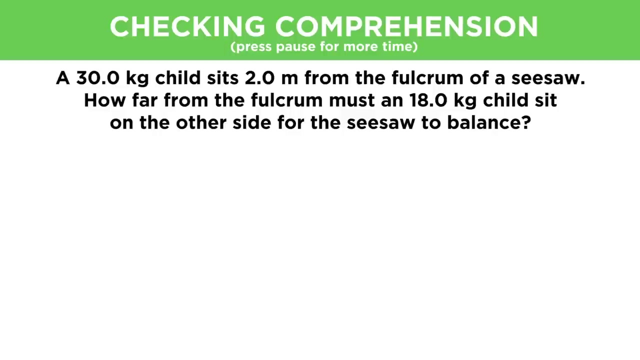